sleek mobile app and hoped to mine the site that people have tuned in with a neat knowledge. Uh, I think when you are using a distributed system like that for upwards of 15 to 20 years, It's not just your theater of money, it's a longer term science and dataavamess. 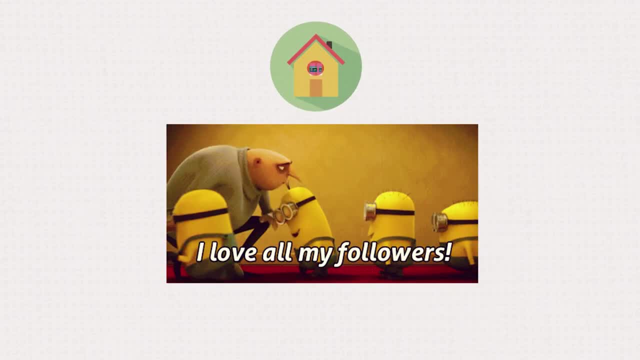 I don't hear much about it because I haven't even seen it myself with that technology yet. Okay, let's put it into a nutshell: I don't actually think it's a small part of a distributed. host it in your machine at home In few months. your service gets popular. your user base grows. 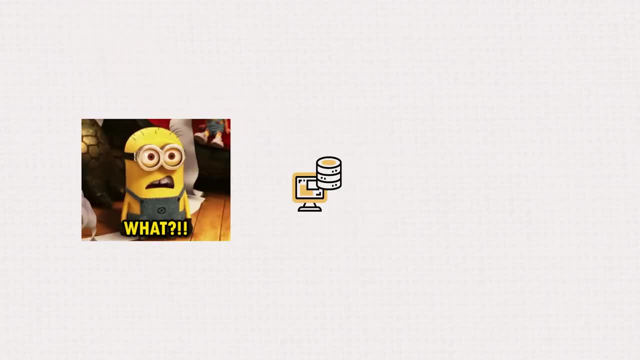 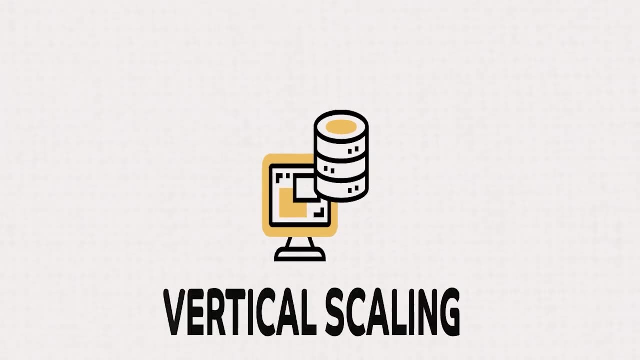 and now your machine can no longer handle the extra load. So you decide to upgrade your computer with new CPU, more RAM, and this is vertical scaling, But it is limited. There is limited amount of memory and computer power you can get from a single machine. So at best you are delaying. 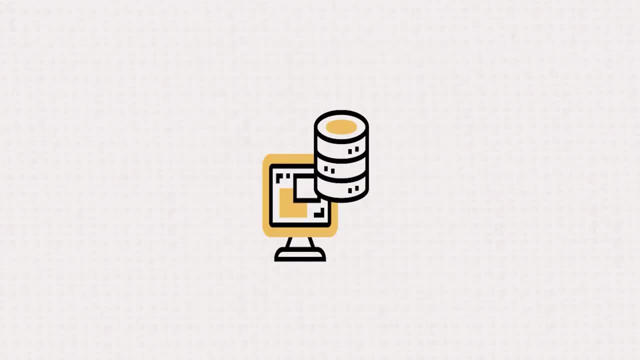 the load issue. Moreover, your computer is single point of failure. if there is a power outage tomorrow in your area, your entire service will go down, And if your users are trying to access your service from other part of the world, most likely they will experience high latency or 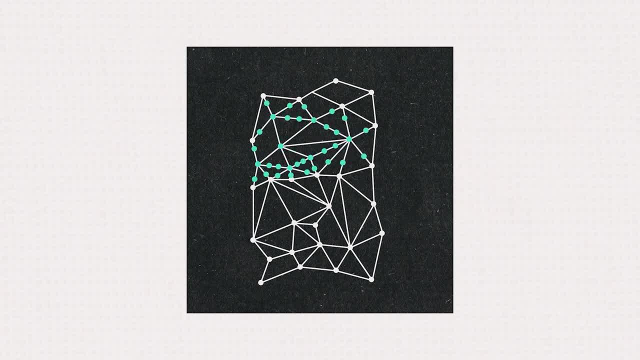 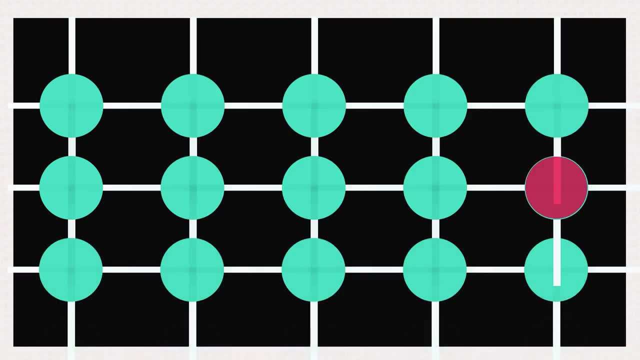 slowness. In contrast, a well-designed distributed system can scale to billions of users. They can scale horizontally and grow or shrink on demand, which takes care of single point of failure and latency issues. A distributed system is a system of several processors running on different computers. 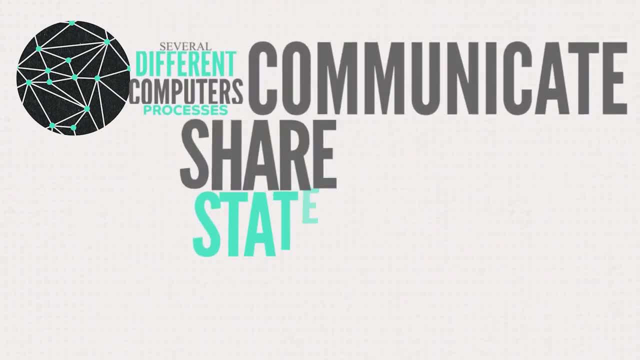 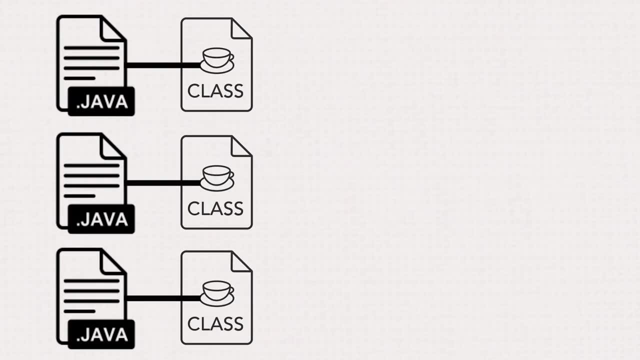 that communicate and coordinate their actions by messaging through the network, sharing a state and sharing data. If you want to know more about this system, please subscribe to our channel. Let's talk about Process. When you compile a Java application, it becomes a class file A. 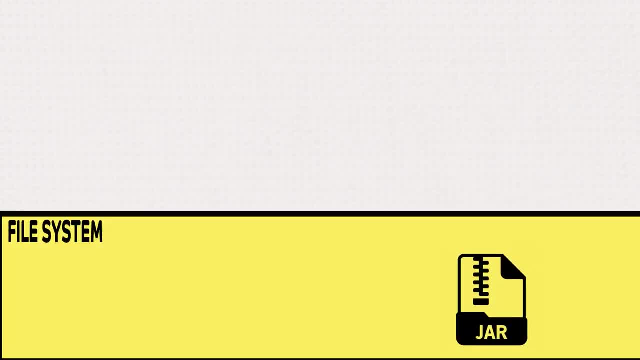 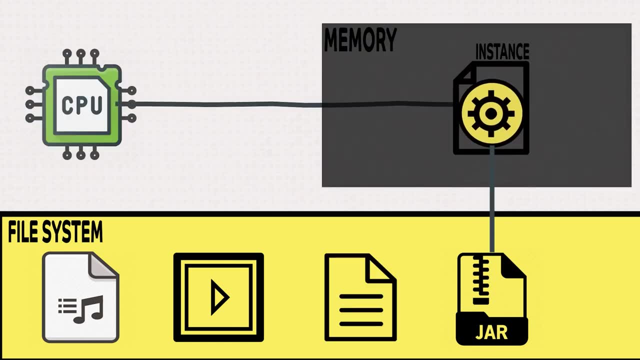 java file is the container of all the class files and this gets stored into your file system just like any audio, video and text files. When you launch the application, the operating system creates an instance of that application in the memory And that instance is 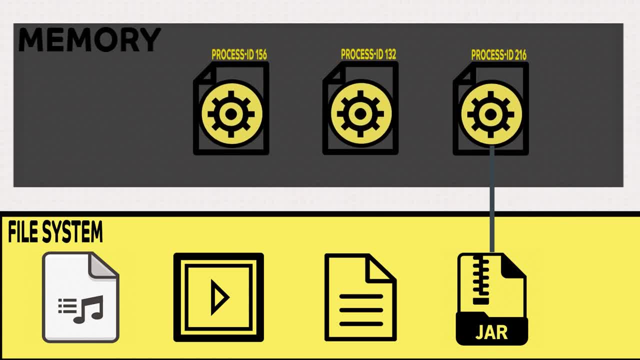 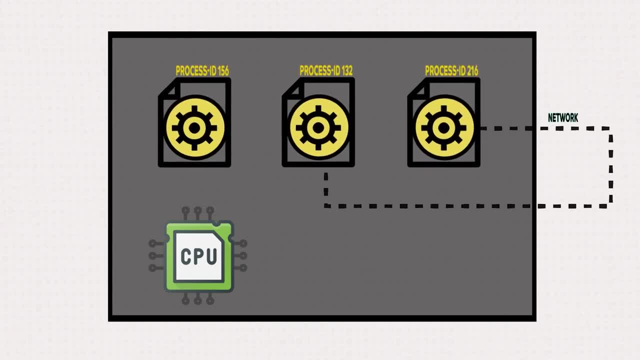 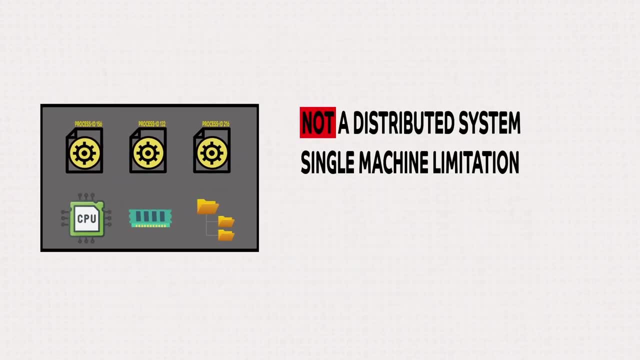 process which is completely isolated to any other processes running in the computer, be it the same application or instances of different applications. Processes running on the same machine can communicate with each other through the network, the file system or the memory, But since it's the same machine, it's not a distributed system. They cannot scale beyond the. 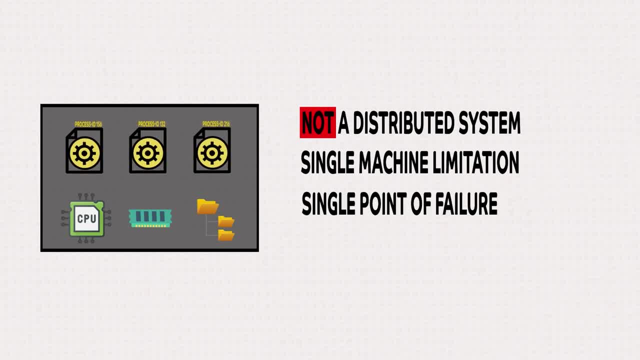 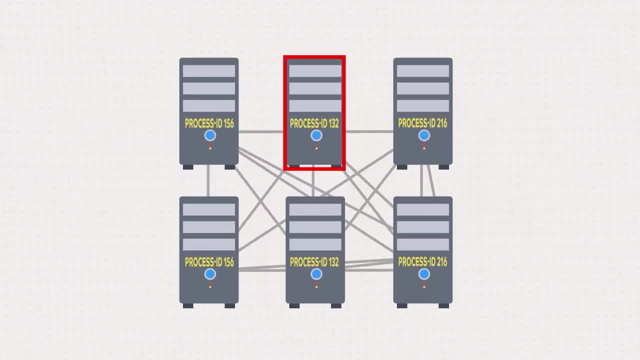 capacity of a single machine and are vulnerable to single point of failure. Now, if you can decouple and put each of the processes in different machines, they can scale horizontally and if any machine goes down, others can take over and maintain availability of your application.